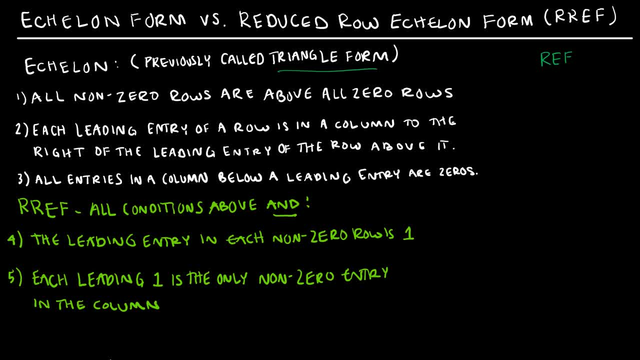 form that we talked about in our last video- and I was talking about Gaussian and Gauss-Jordan elimination In echelon form: all non-zero rows- and up to this point we haven't had any rows that were all zeros, but sometimes you do So all non-zero rows are, above all, zero. 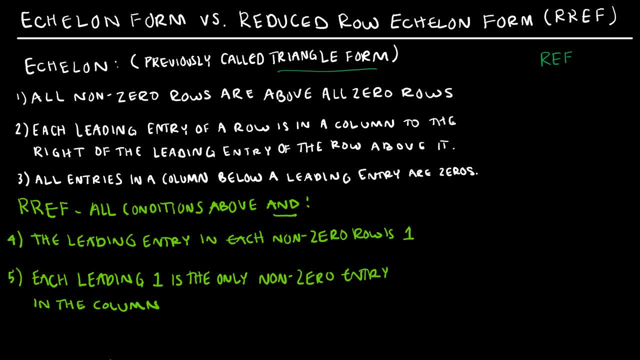 rows. So all non-zero rows are, above all, zero rows. So all non-zero rows are, above all, zero rows. Each leading entry of a row is in a column to the right of the leading entry of the row above it. and again, that's why it was triangle form, because, as we were writing this, let's say, I had 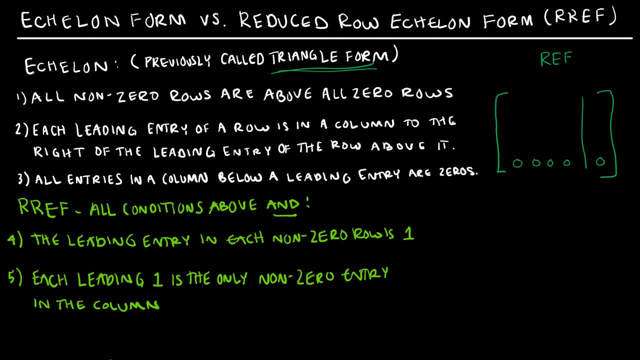 this would be a zero all zero row. that would obviously be near the bottom or at the bottom. If you had more than one all zero row, they would all both be on the bottom or all. So, for instance, I could have something like two, seven, six, three, two, zero, because we talked. 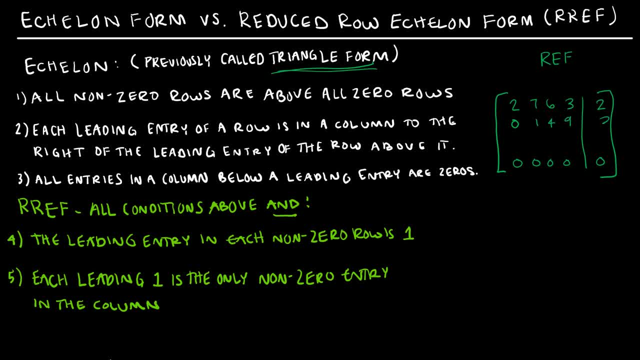 about needing that zero, one, four, nine, three, and then I might have even three zeros and a seven and a six. This would be an echelon form, and again it looks kind of like triangle form that we talked about before, And again, all entries in a column. 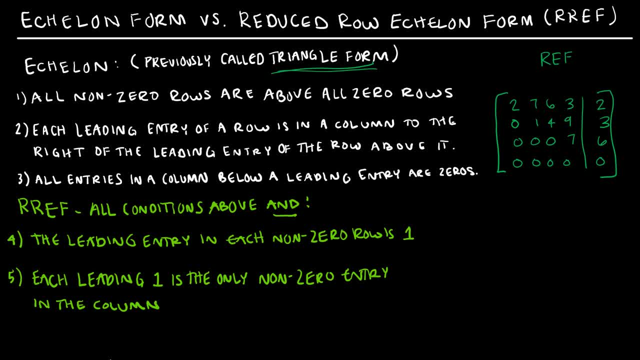 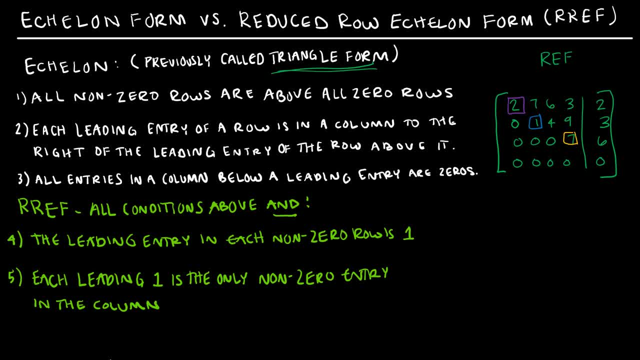 and all zeros below it, And all of those rows, as we can see, cascade down to the right. That is called echelon form. If we want reduced row echelon form, then each leading entry in a non-zero row is a one, And so in our last video I kind of did that, naturally. 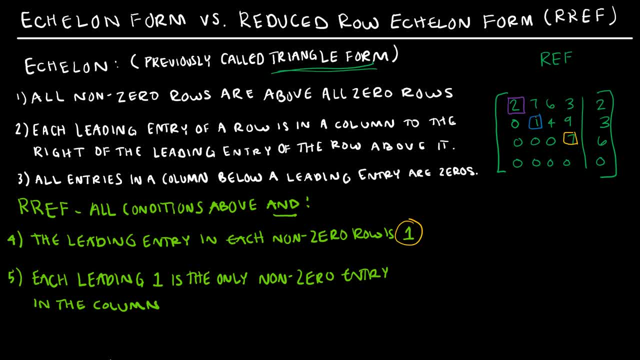 as I turned them into ones just because they were easier, And each leading one is the only non-zero entry. So essentially what we're saying is: I've got a one here and that's the only value on the coefficient side of the matrix, So obviously I can have something else on the right side. 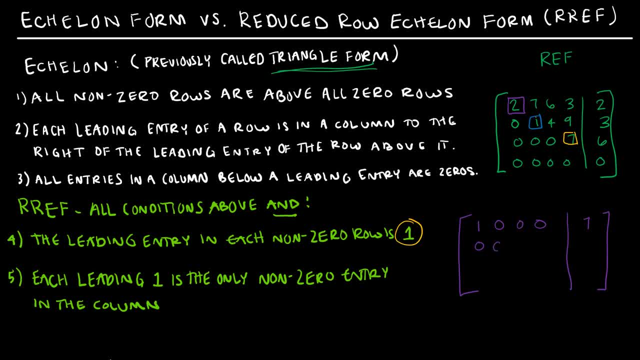 which is the solution. I might have a couple of zeros and then three, not three. it has to be a one One zero four. And then, remember, this would be illegal because they're not cascading down to the right. So I would. 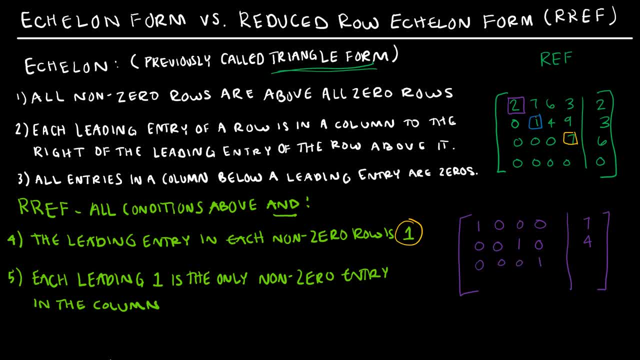 have to have swapped those rows. I can have a one here and then I still can have an all zero row. So that's an example Of reduced row echelon form. It has all of the same things that echelon form has, but all leading entries are one and all non-ones are zeros. 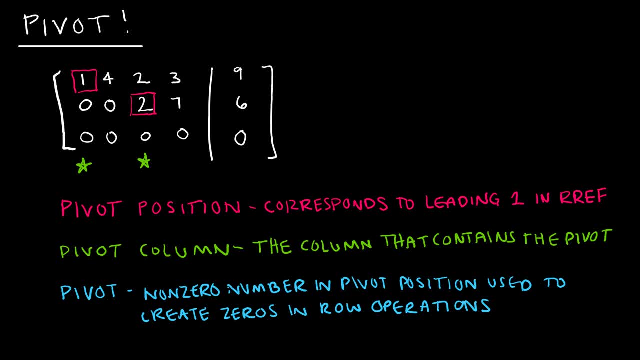 Pivots. What are they? What do we need them for? Well, a pivot you're going to hear quite often, and it's just terminology that tells us that we're looking at that leading coefficient in the row. So previously, when we talked about echelon form or reduced row echelon form, a pivot position corresponds to where the one would be in reduced row, echelon form or essentially what's the leading value. So here the leading coefficient is one. 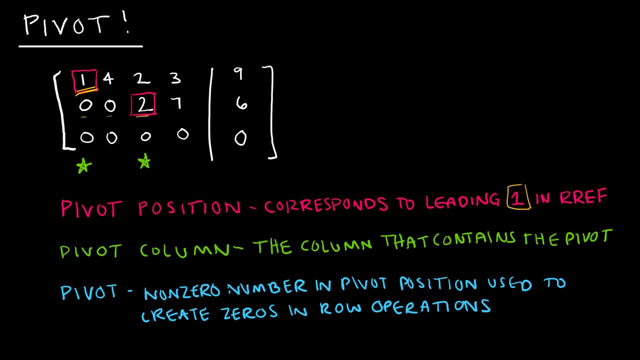 And here notice we've got zeros beforehand, so the leading coefficient is two. Those are pivot positions in pink. The pivot column is just the column that contains the pivot Position, And then a pivot is a non-zero number in the pivot position used to create zeros in your row operations. 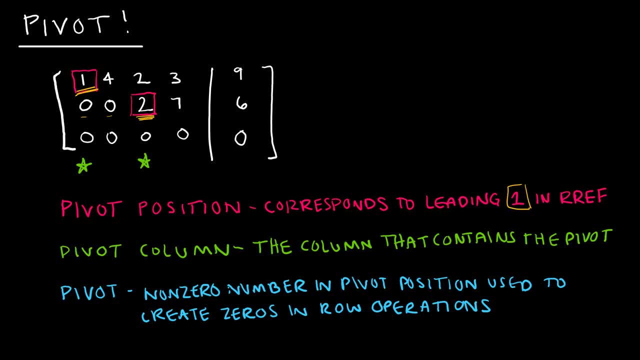 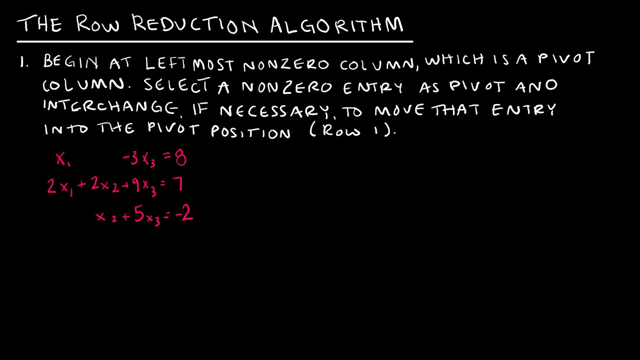 So what we're going to do now is we're going to use these pivots and use the essentially the same steps we were looking at in the last video, but we're going to solidify what those steps should be, Which is, of course, the row-reduction algorithm. 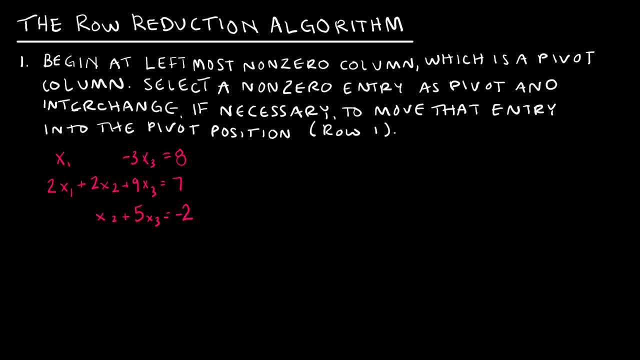 So the algorithm will essentially gives you steps to follow in order to find the solution in the easiest, fastest way possible. so the first thing you should do, of course, is to write it as a augmented matrix, which I didn't add that as a step, because honestly, I shouldn't have to. so let's write that quickly. 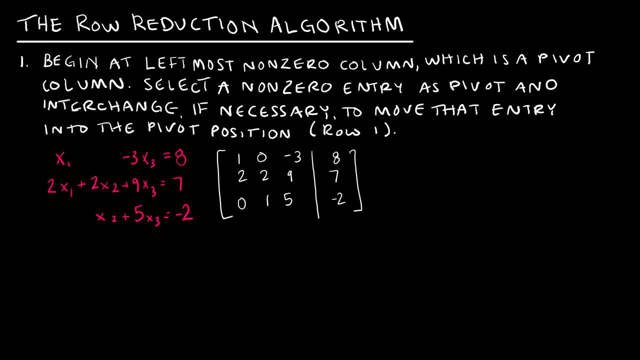 and my algorithm says: begin at the leftmost non-zero column. so that's code for start. right here. that's a pivot column. select a non-zero entry as the pivot and interchange if necessary to move that entry into the pivots position, which is row one. so we really want that first left-hand top row to be a pivot. 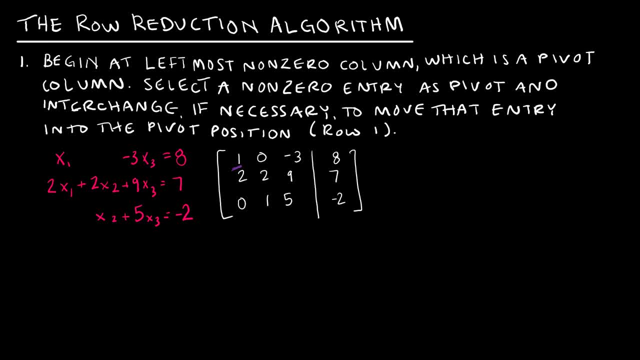 and the only time that's not going to be a pivot is when there is no value in the first column, which really would never happen, because if there wasn't a value in the first column, we just wouldn't have the first column. it would start at the second column. so I don't have to do step one because I 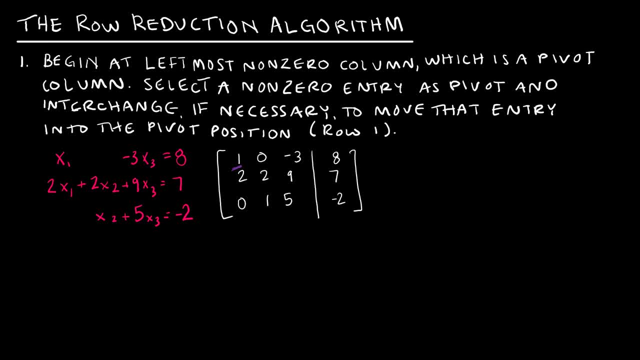 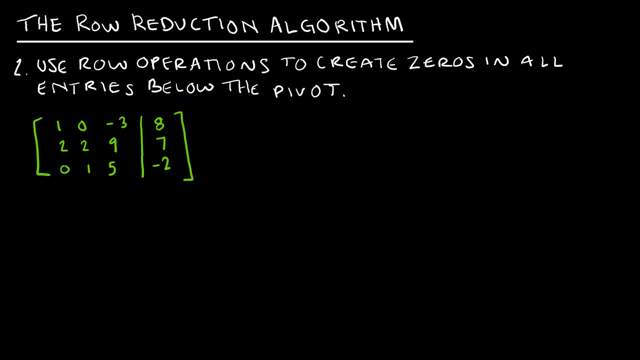 already have a one exactly where I want the one. however, let's say this guy was my first row, then I would have to do a swap in order to get a one into that first position. step two in our algorithm is to use row operations to create zeros and entries. 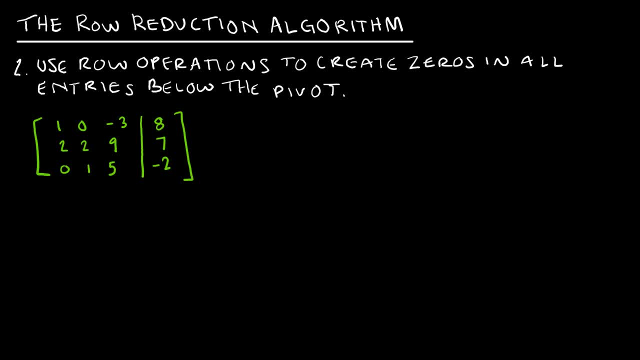 below the pivot. so here's my pivot. I want to now create zeros here and here. now, as we can see, I'm pretty fortunate. I already have a zero in row three. to get a zero in row two, I would need to add negative two to positive two, so that's. 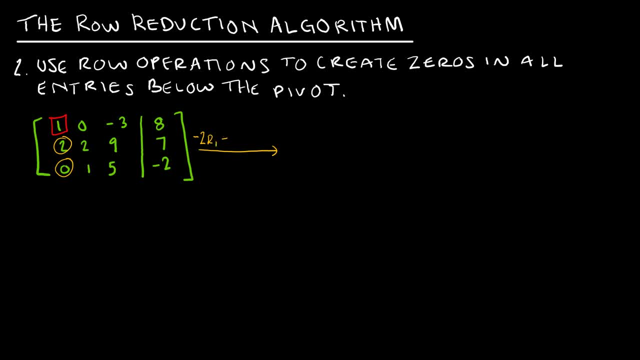 exactly what I'm going to do. I'm going to take negative two times row one and add it to row two, and that's going to be my new row 2. now, again, we're doing a lot of mental math here, but if you need to, you can feel free to go ahead and write. 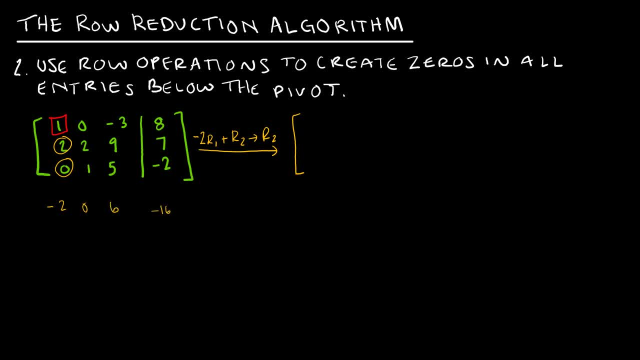 the negative two zero six negative 16, to help you in your calculations, because I'm going to be adding that to row two from my new row two. so row one is going to remain the same, 3 is going to remain the same and row 2 is going to be 0,, 2,, 6 and 9, and then negative. 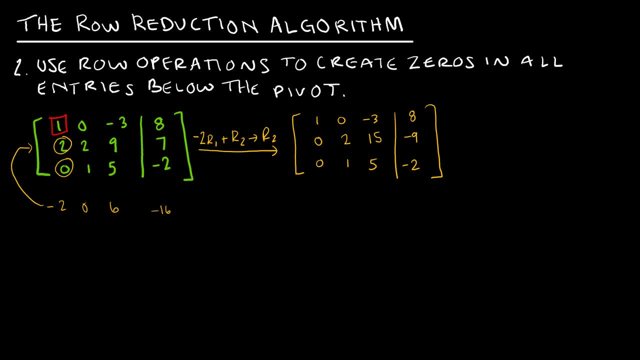 16 and 7.. So that is step 2, is again to get zeros where we want them and, as we can see, we did get zeros where we wanted them. Step 3, repeat this process for the remaining rows, ignoring rows you've already applied. 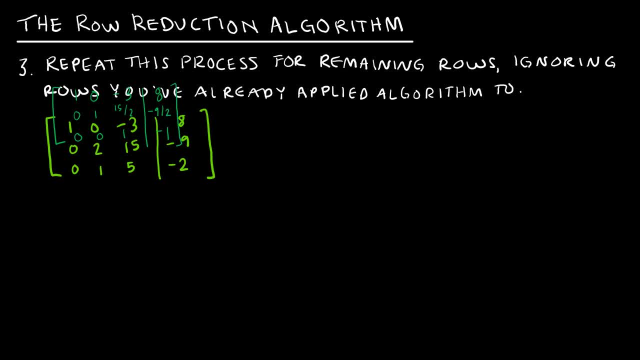 the algorithm to, and that means the process was get this to be a 1 and then get zeros below it. So that means my next step is to get that 2 to be a 1.. So let's do that. How am I going to make that a 1?? 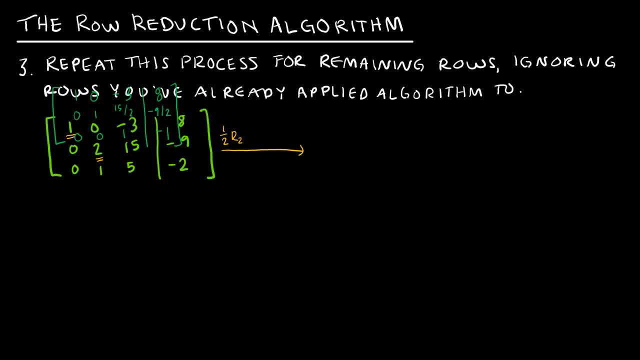 I'm going to take half of it. Half of row 2 will be my new row 2, which means row 1 remains the same and row 3 remains the same and row 2 is half and again. decimals or fractions doesn't matter to me, as long. 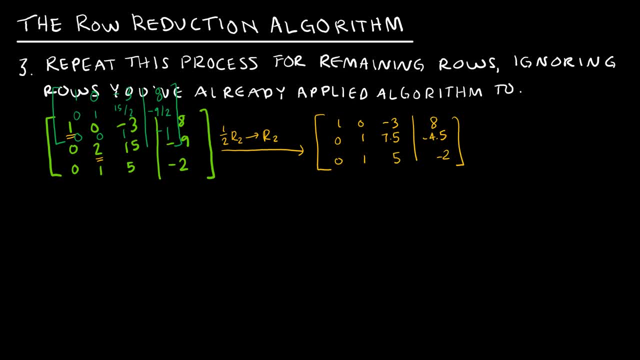 as the decimals are exact. And then how am I going to get a 0 below it? I'm going to have to add them. So I'm going to get a 0 here next, and to do that I'm going to take negative row 2. 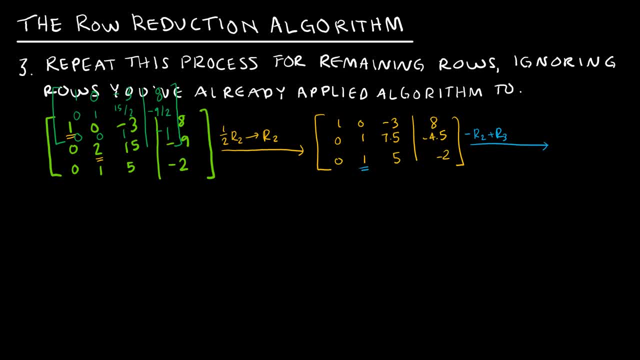 plus row 3, to be my new row 3, which means row 1 remains the same, row 3 remains the same and row 2 is going to. oh, just kidding yikes. Row 2 remains the same. 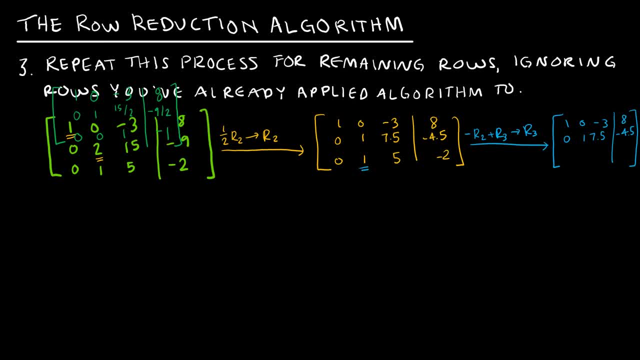 And then row 3 is negative, row 2 plus row 3.. So negative 0 plus 0,, negative 1 plus 1, that gives me the 0 I wanted. negative 7.5 plus 5.. And negative negative 4.5.. 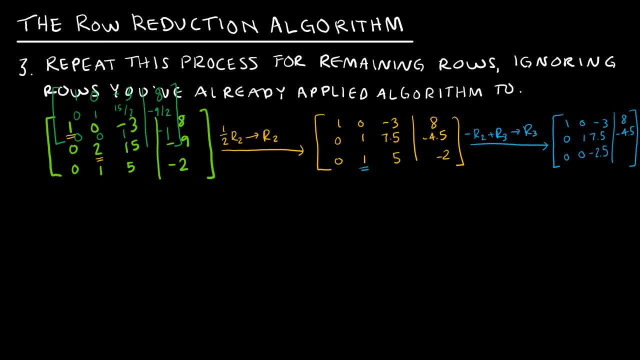 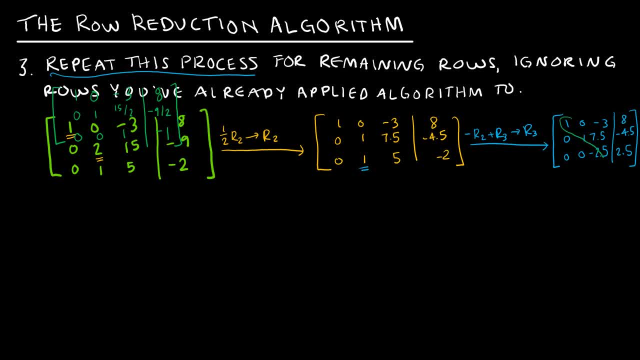 I'm going to keep doing that until I get all 1s, which I don't have yet. So how am I going to get all 1s? I'm going to take, And again, this is why it is better to write these as fractions. 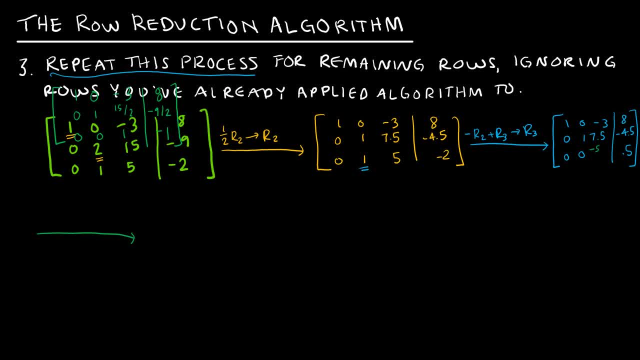 So that was negative 2.5, which is negative 5 halves, And this was positive 2.5, which is positive 5 halves. So how am I going to turn that into a 1?? I'm going to multiply by negative 2, fifths row 3 to be my new row 3.. 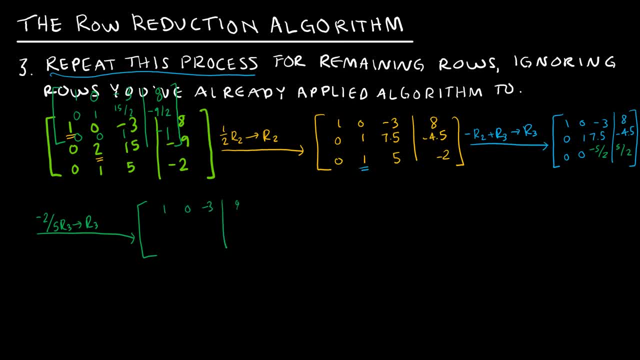 So row 1 remains the same. And again, this is why it is better to write these as fractions. So I'm going to take- And again, this is why I'm repeating the process over and over: Row 2 remains the same. 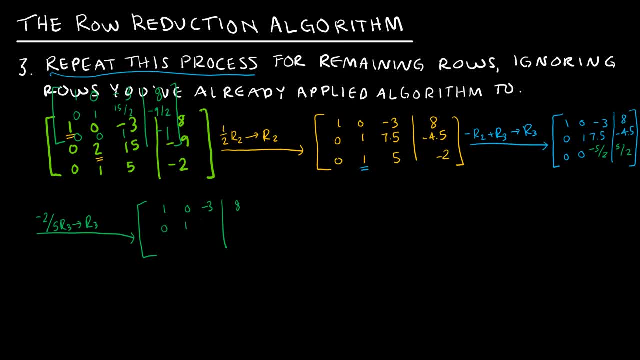 I'm going toô Write this as I'm going to write it as A divisor And again, this is where I'm going to И A divisor. So row 2 remains the same: 15 halves and negative 9 halves. 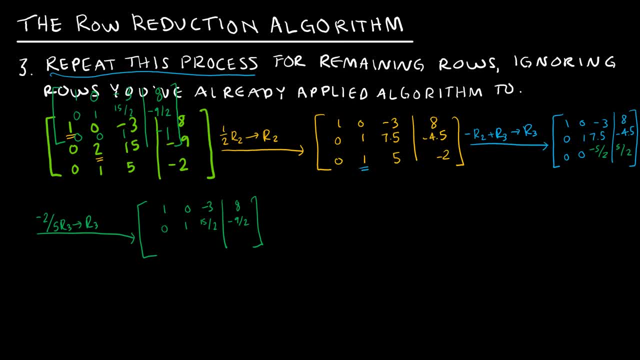 And then row 3 is essentially multiplying by the reciprocal- sorry, by the negative reciprocal, which gives me 1 here and negative 1 here And again. we've repeated the process for everything. So we've talked before about how you can stop here, and if I stop here, that is going to give me a back substitution situation. but I want to have reduced row echelon form, so I want all of these guys to be zeros as well. 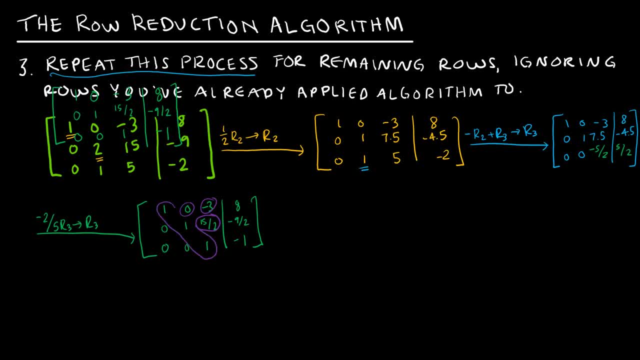 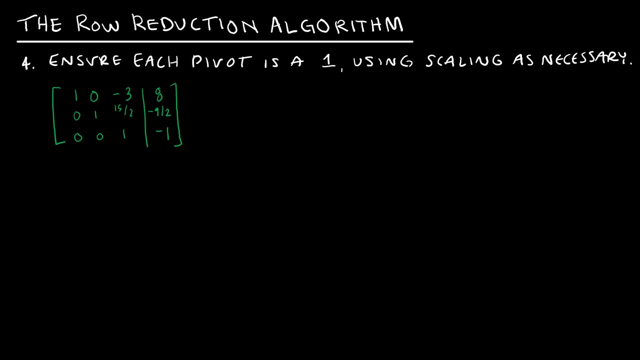 So remember reduced row. echelon form has ones here and zeros everywhere else, or we could have an all zero row. Step four is essentially to ensure that each pivot is a one, So the way that I just naturally do this is I always turn them into a one, So I could have not used that as part of my process in steps one through three. 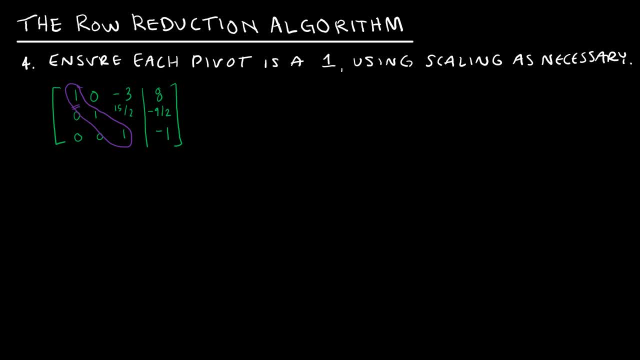 I could have. I could have just ensured that I have a value where in a pivot position, and not necessarily that that value was one. So I automatically just get that value to be one. So I really don't have to do step four, because I wrap step four into the first three steps. 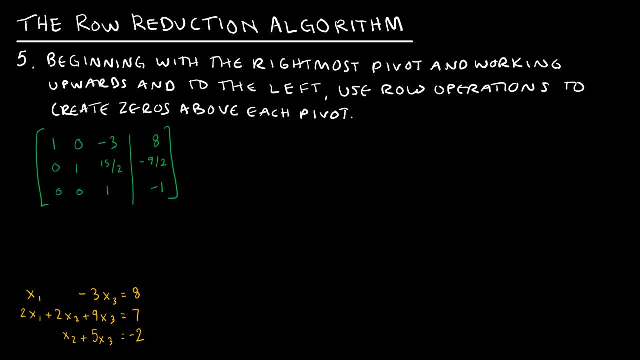 And for our final step again, we already have ones exactly where we want them here, and we have all of our zeros here. Our final step, Our final step, is to turn zeros, excuse me, to turn these values into zeros, So everything above the diagonal of ones. So to do that, we're going to start working upwards and to the left, which means I'm starting with the rightmost pivot, which is the bottom one, and I'm going to work upwards and then to the left. So I'm going to start here with 15 halves. 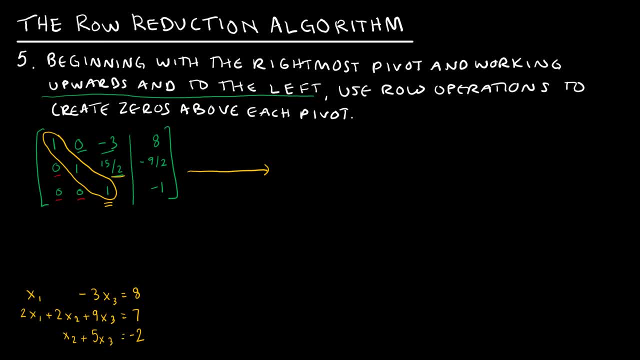 How do I turn 15 halves into zero? I'd have to add negative 15 halves. So that's what I'm going to take times row three to get my new row two. So I'm adding negative 15 halves times row three to be my new row two, which means row one is the same And row three we don't want to touch because we have it exactly where we want it. 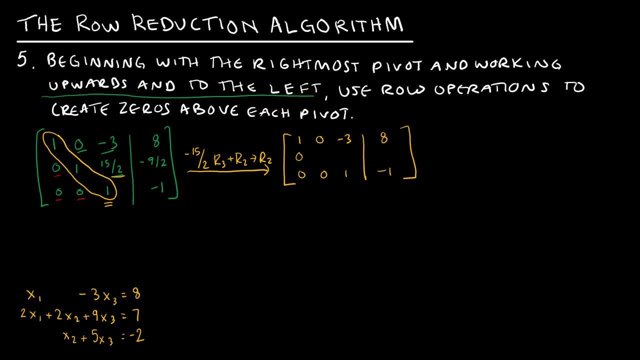 If I take negative 15 halves times zero plus zero, and then of course zero plus one, negative 15 halves plus 15 halves gives me zero, which is of course the whole point. And then negative 15 halves times negative one is positive- 15 halves plus negative nine halves gives me six halves or three. 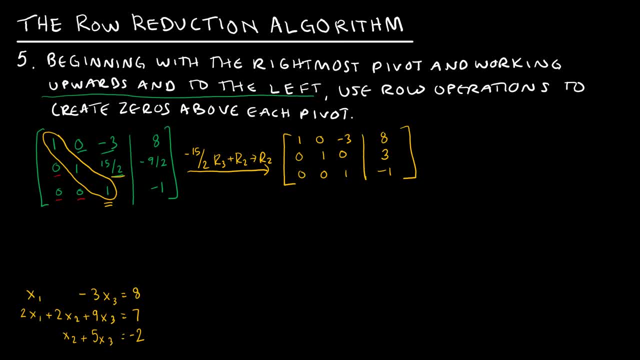 Now from here I would work upwards and to the left, And so again, that means this guy now has to be zero, and I don't have to worry about this one because he's already there. So my last step is to turn negative 3 into 0.. 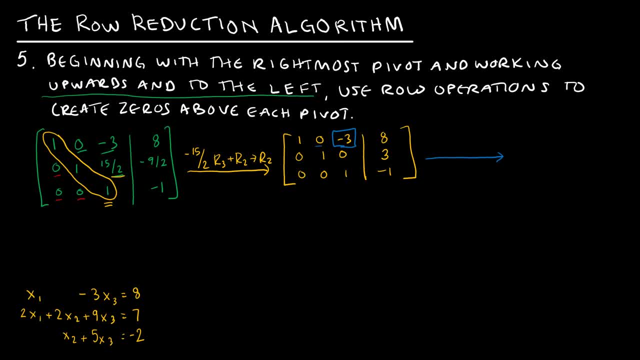 How do I turn negative 3 into 0?? I add positive 3, so I'm going to take 3 times row 3 plus row 1 to be my new row 1, which means row 2 is perfect just as it is. 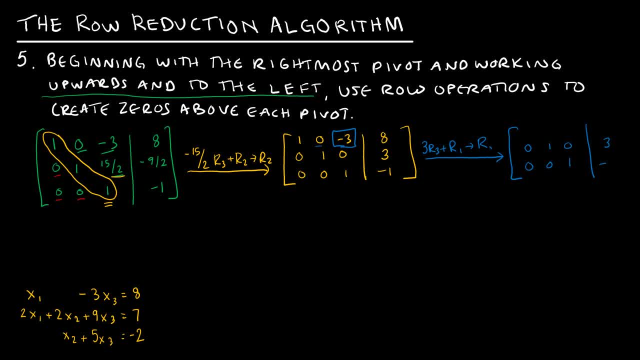 We're not going to touch it. Row 3 is perfect just as it is. We're not going to touch it. Row 1 is 3 times row 3 plus row 1, which gives me 1 here, 0 here, 0 here. 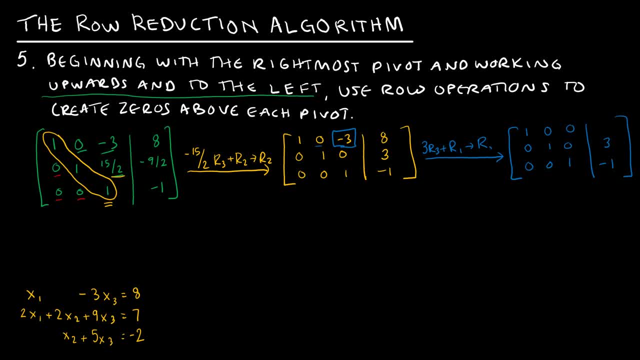 And then 3 times negative. 1 is negative. 3 plus 8 gives me 5.. So that tells me that my solution- remember what this means is- I have- 1x1 is equal to 5.. This one tells me that 1x2 is equal to 3.. 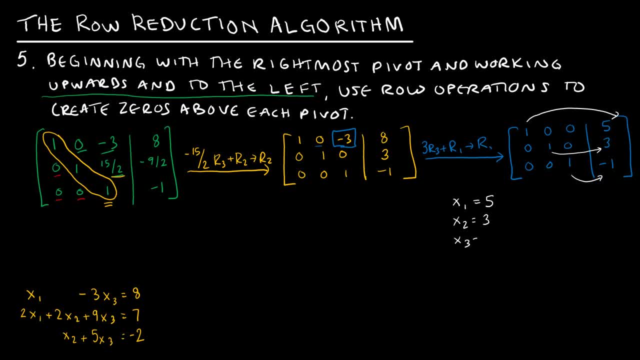 This one tells me that 1x3 is equal to negative 1.. So my solution is 5,3,, negative 1.. Now in the last video, when we didn't go through the algorithm but essentially we followed these steps, 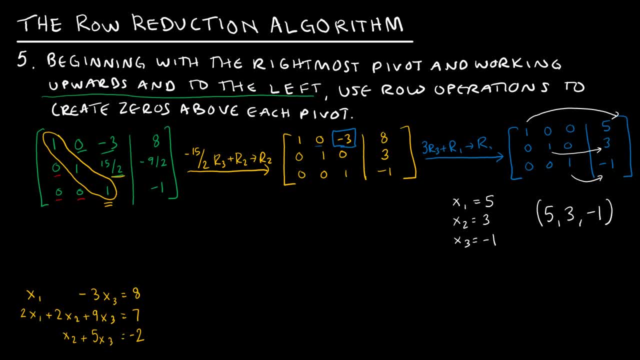 we never really checked our answer, But keep in mind, if you do solve a system, this should work in all of these equations. And notice that I've just rewritten them down here, So I should be able to replace x1 with 5 and x3 with negative 1.. 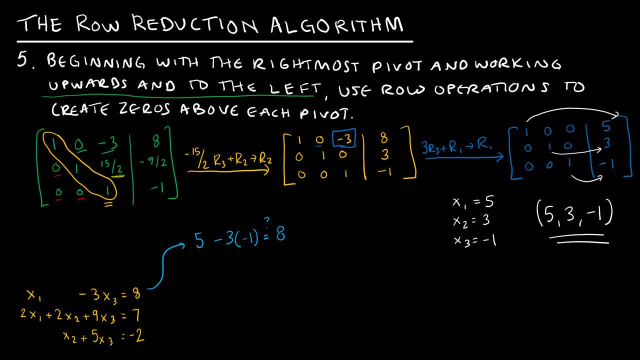 And that should equal 8.. So 5, this is plus 3.. Does 5 plus 3 equals 8?? Yes, whoops, 8 equals 8, check, check. So it works for the first one. Does it work for the second one? 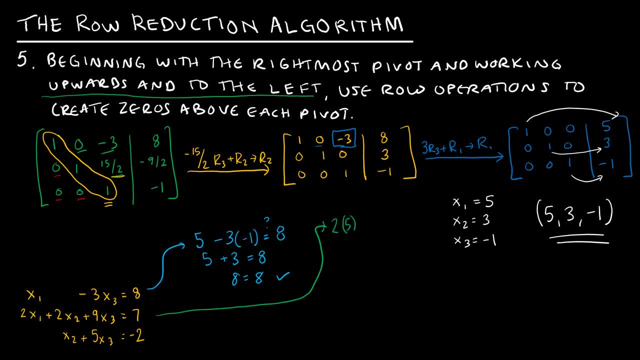 That's telling me 2 times 5 plus 2 times 3.. Plus 9 times negative 1, does it equal 7?? So that's 10 plus 6 plus negative 9, does it equal 7?? 10 plus 6 is 16,. 16 plus negative 9 is 7,. 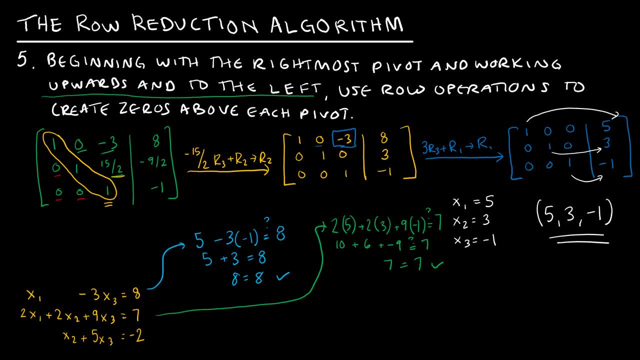 so I have 7 equals 7, and it works. And of course then I would also check the last one, which says x2, which is 3 plus 5 times negative 1, does it equal negative 2?? 3 plus negative 5, does that equal negative 2?? 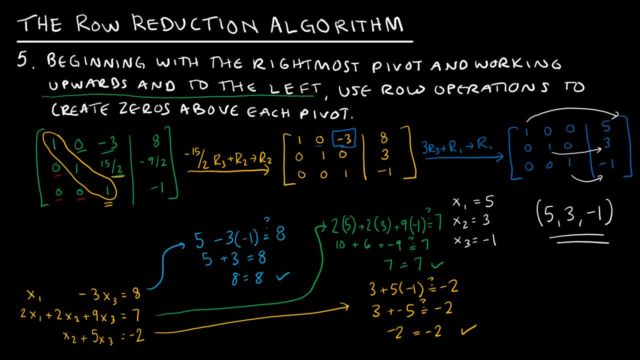 Negative 2 equals negative 2. And so, again, I'm just that much more confident that my solution is correct.